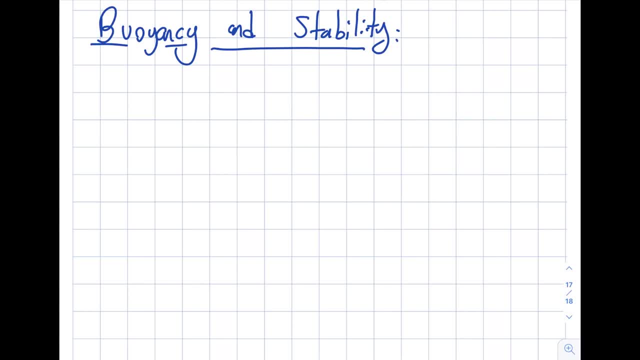 go ahead and see the principle that I'm going to introduce. It's called Archimedes. Good luck spelling that out as well. The rest will be fine, okay, So let me write what I just said- Well, not the spelling part. Why? this is what I'm going to answer: fully submerged, or let's call this partially submerged bodies- float. 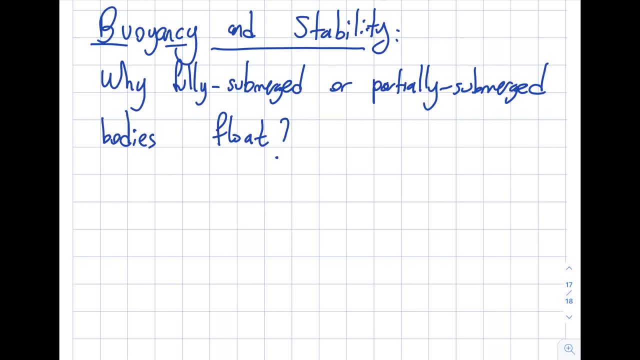 Okay, let me answer this in this way. Let's have a free surface over here and I have- I don't know something like this- a box, rectangular cube, rather right, I'm drawing in 2D, So this is y. pointing up is z. 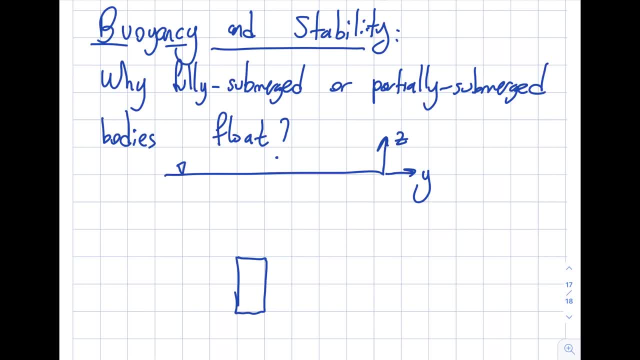 Okay, so what will be the net force on this? okay, So it may look unconventional that it is actually the force is going to go up, because it's kind of like the opposite to salt mechanics, right, If I leave something usually. 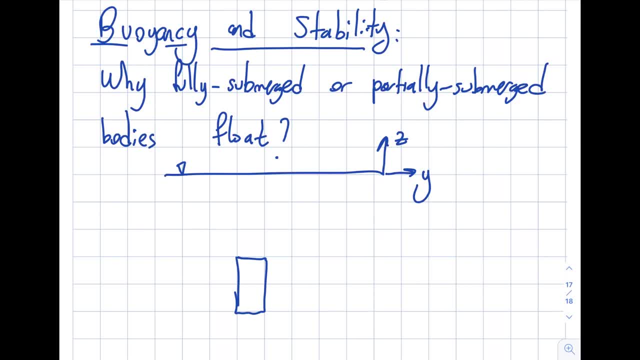 it goes down in the negative z direction, but I'm saying that this is going to go up, Why? Well, let me explain. okay, I need to call a few height dimensions, So let's call this h1, and let's call this h2, okay, So now let's look at the pressure distribution on the right. 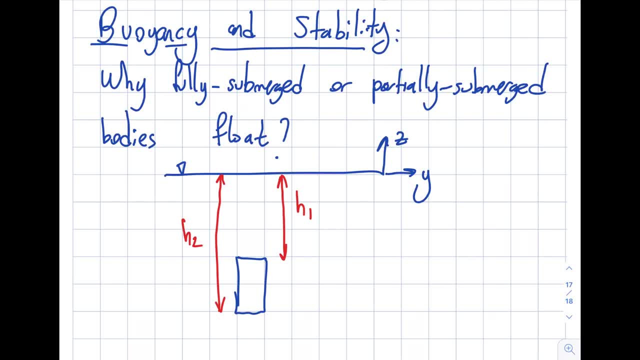 and on the left of this cube. You may realize that the pressure is going to start from here and then it's going to go down. It's going to increase linearly, right, it's gonna increase linear, like this as well. so, if I look, 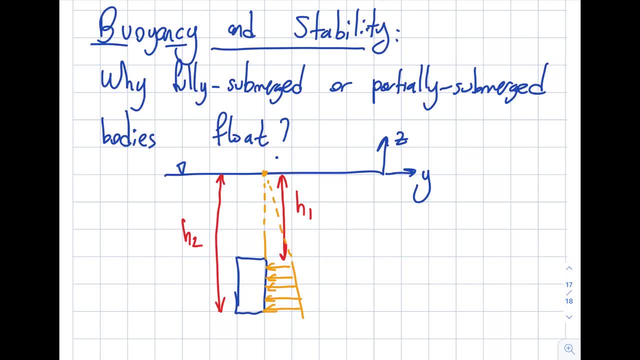 over here. you will see that this will be the force, or rather the pressure distribution on that face. so if I do a similar analogy on the other side, you will see that. well, I hope that my slope is the same, because that's what I'm trying to show you now. okay, here we go again. the right and left is not the same. 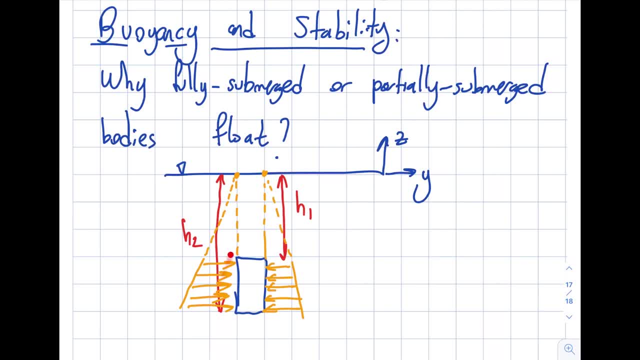 this looks bigger, but the point is in reality: as the slope is the same, the height is the same. let's say, I pick an arbitrary height over here, the pressure over here will be pushing this way, the pressure over here will be pushing with this way and the magnitude will be the same. so my point is that 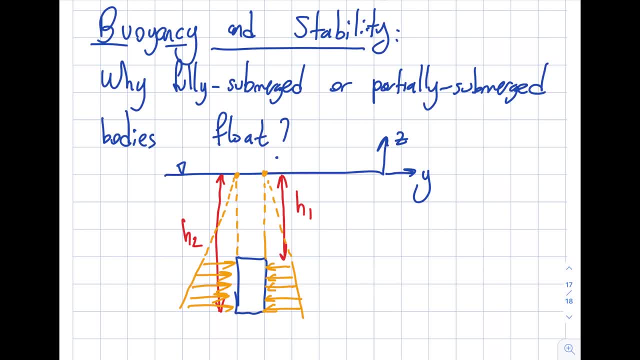 they will cancel each other right and left, it will be quite stable. I'm good to go. how about the top and the bottom? and that's where it gets into the buoyancy force. so on the top, let's say that, remember, pressure always pushes it in right. 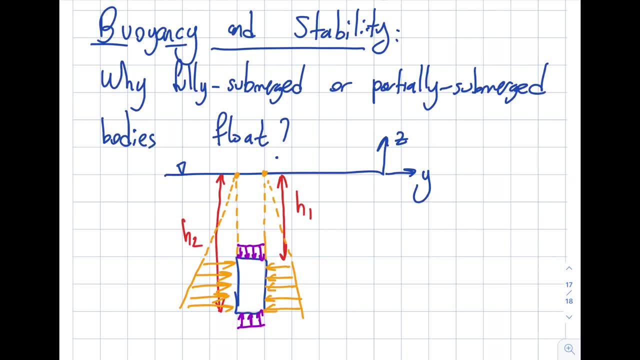 it's pushing, it's not, it's a compressive right, it's positive. so then let's, let's go ahead and calculate this. so this will be well, Rho G, or I can call the specific weight right times, h1, that's the pressure, and actually 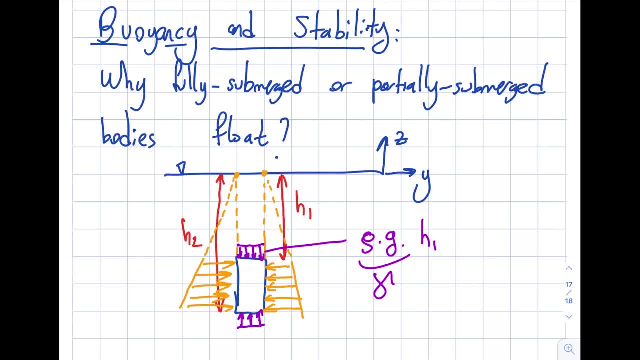 uniform right specific weight of whatever I'm traveling in times. the h1 will be the pressure, not the force pressure pushing it down. and if I multiply this by the area, and the area is basically, let's call this W, which is the width of this, and I'm gonna call this D. D is into the page or into the screen in this case. so 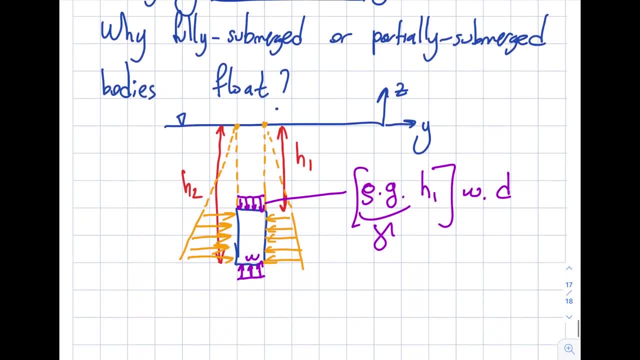 that's the depth into the page. okay, all right, that's fine, let's do the same analogy for here as well. so what will happen here is Rho G times h2- right, because I'm h2 from the free surface and area will be the same. you can see that. 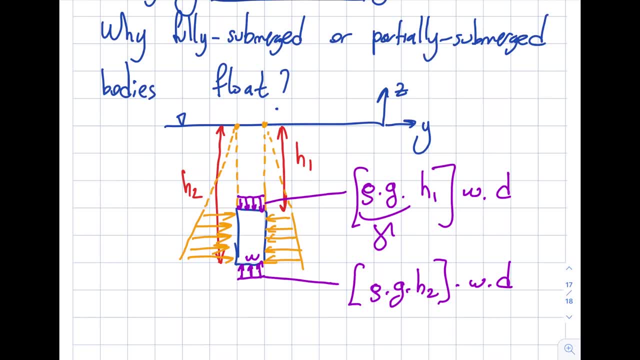 the width times into the screen depth? okay, all right. so my question is: look here. so these are multiplying both Rho G is constant or specific weight gamma is constant. so you can see over here: so this is h1 pushing it down and this is h2 which is larger. you can see with the 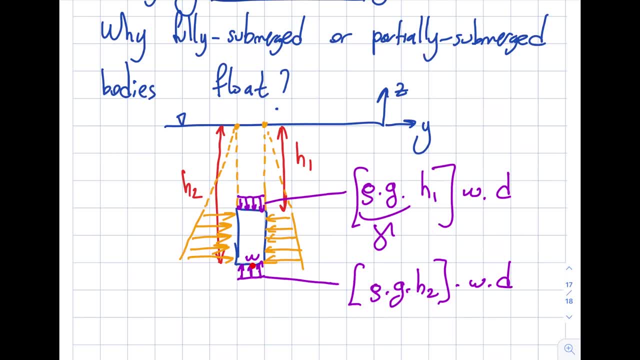 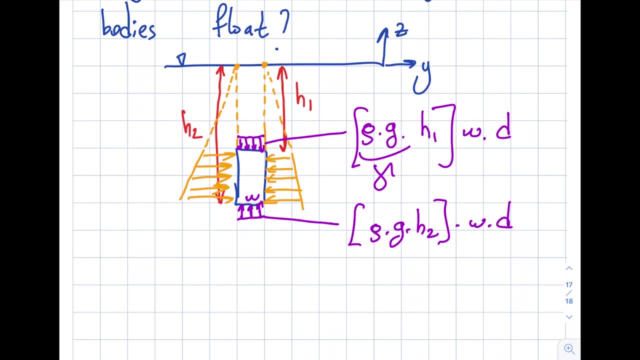 red font over here. so basically, this is pushing this up more than this is pushing it down, right. so then this is gonna go up because there's a more force in the positive Z direction. let me see whether I can get a formula here. that would be nice, because I want to talk quantitatively, not 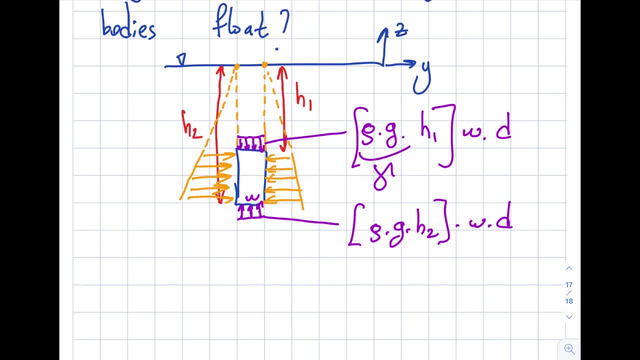 qualitatively. you know what? let me you know. one is push. this is pushing it up, this is pushing it down with a lower amount. so let me get the net force from this angle. so, in order to do that, you can see that this is aligned with the 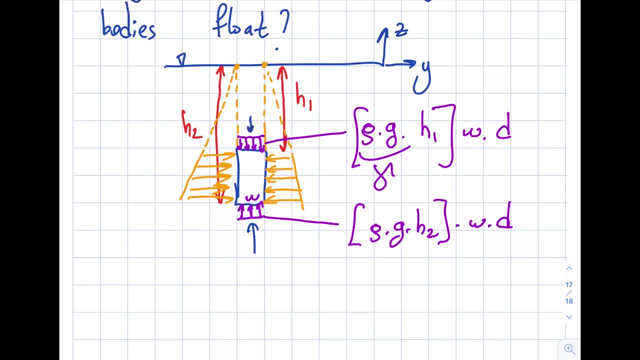 positive Z, this is aligned with the negative Z. that's why I'm gonna write it this way: specific weight times h2 W. width times depth minus specific rate: the same specific rate h1 W D. right, so you can see these three terms are common, so I can get myself: specific weight W D times h2 minus h1. 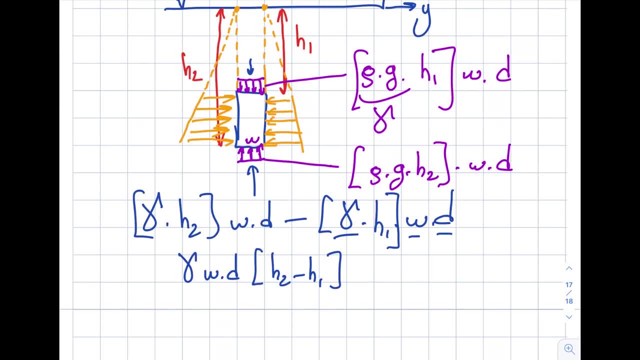 right. so what is h2 minus h1? it's right here. right, that is the H H of this block. okay, so what I get myself is specific weight times, W times, D times H. what is W times D times H? well, that is the volume of. so then, as you can see in here that I get, 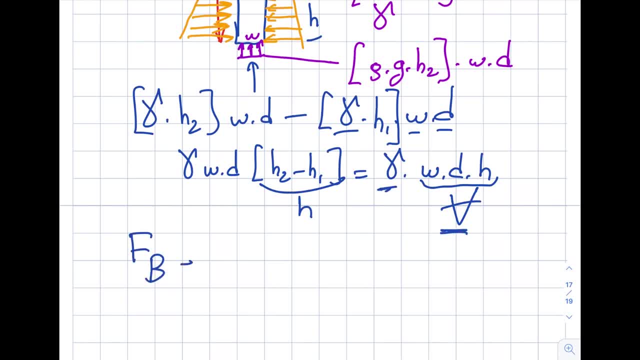 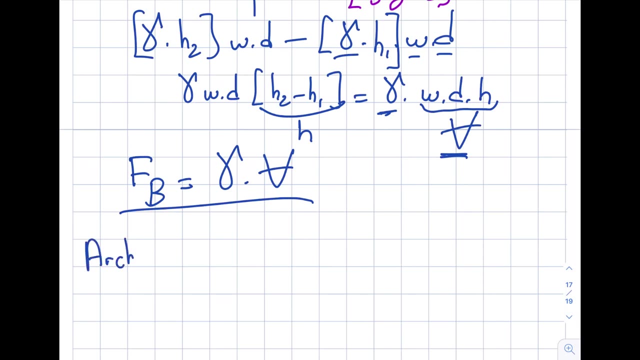 myself a fairly nice equation. so, as you can see here, this buoyant force becomes specific weight of the fluid times, the displaced volume. okay, you can see from here. we derived it for you. but if you want to write it basically, what I just said is the Archimedes, it's a Greek scientists principle, basically what he 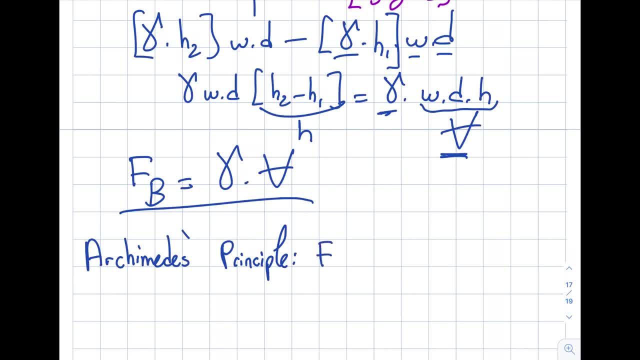 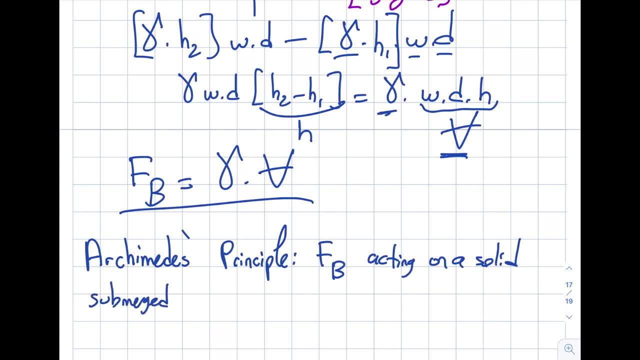 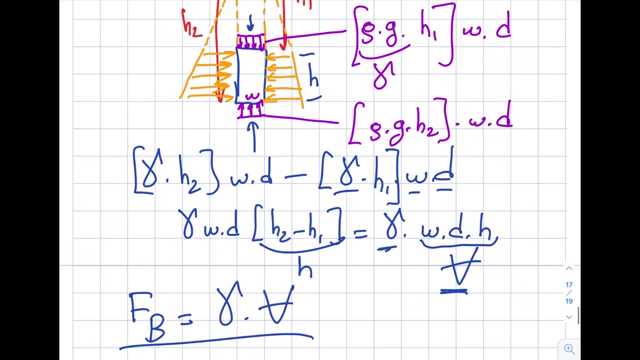 submerged or partial submerged fluid is equal to weight of the. so something in here that this- this terminology is used a lot in this buoyant force displaced fluid. what I mean by that is this: so think about it. so I I'm inserting this box over here, so if this box was not there, this whole thing was. 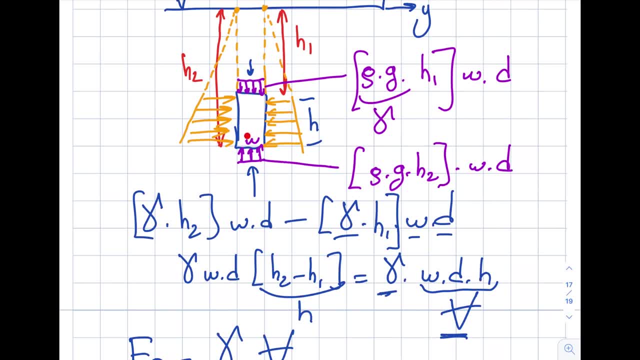 occupied by the liquid that I have in this particular case. right, so this is now this place, so this is gone away. I don't have any more water over here. is this a solid? that's what they mean, so it's offensive way of saying that this is. 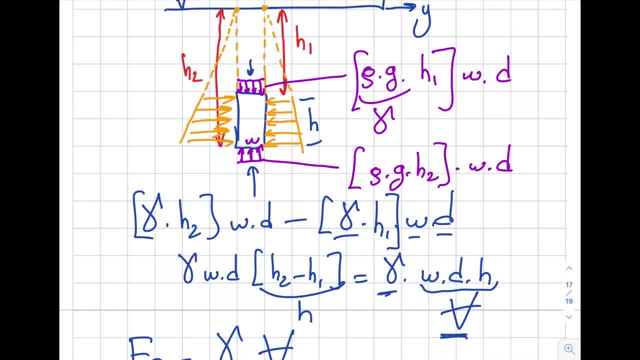 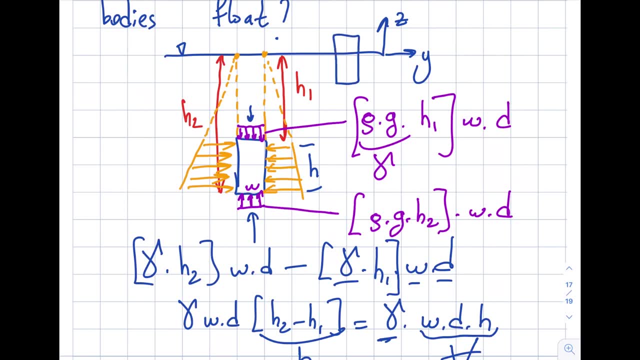 the volume of it. all right, we get to the bottom point, which is that this is the. the thing, though, important is if this is partially submerged. so let's say that over here I have a box like this, right, so in that case, this place. weight of the. 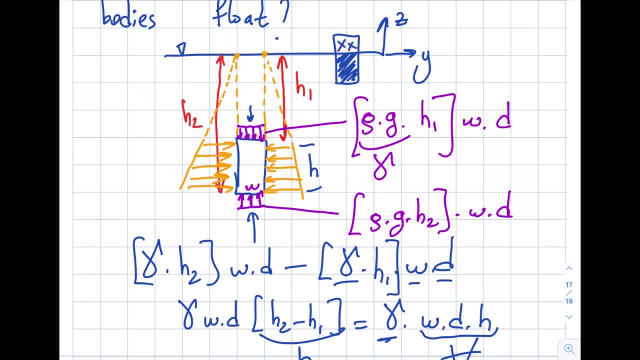 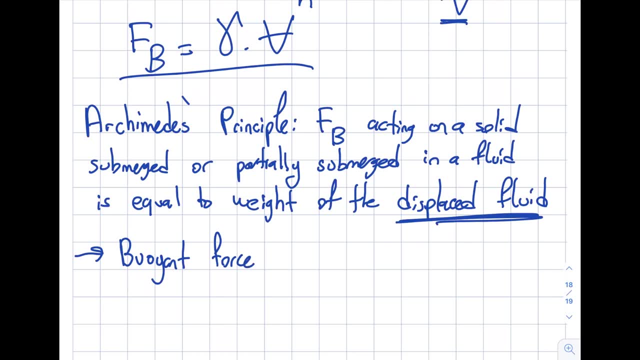 fluid will be only this. you're not going to include that part, okay, because that's not really what I'm after. buoyant force passes through the centroid of the displaced volume. okay, you can see now. we displaced fluid, displaced volume. you see what I mean. we tend to. 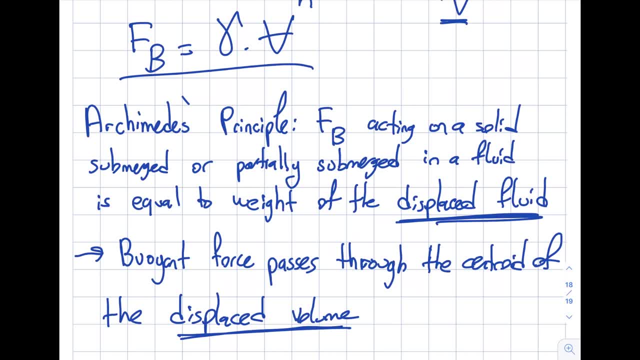 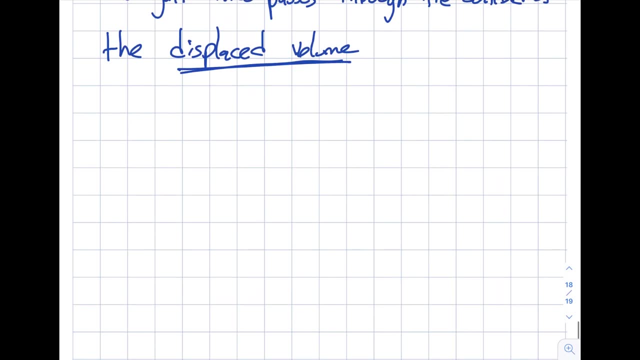 use this place often, okay, and this is called the center of buoyancy. you can guess this one as well. okay, so this is important. this can be the same point as the centroid. this can be completely different, okay, so now let's talk a little bit about the hydrodynamic, the stable or non-stable. so what I want to? 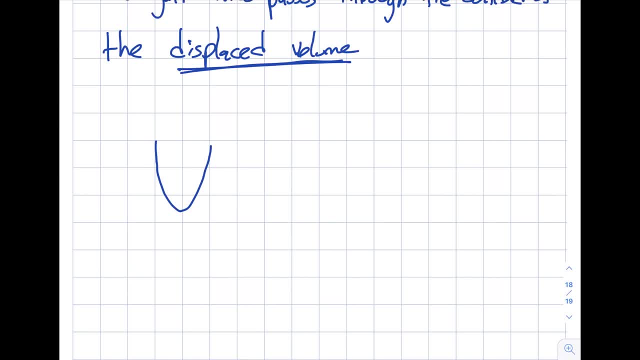 do is, let's say, my drawings are not the best, but I'll do so. I have kind of like a ship over here, okay, so this is the. you know, actually it's not too bad, right? so this ship is continually stop, and right, then this is the number one. 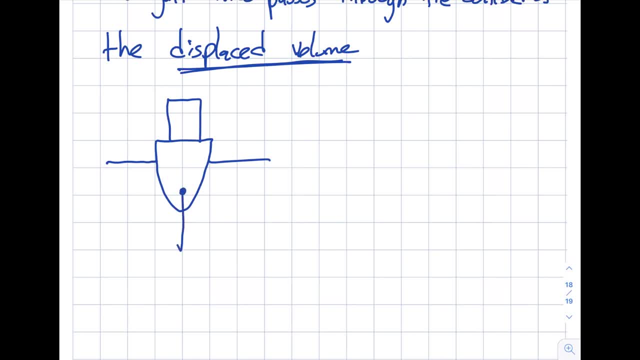 so let's take a look at it. if my weight is down here, right, let's say that I'm on carrying oil over here, okay, it's full. so what will happen is the weight will be down here. the buoyant force will be like this: it will be about the weight. so 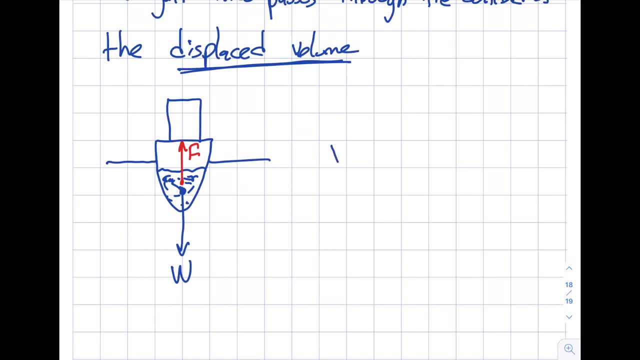 what will happen is, let's say that you know, with the wind and all my ships gets some angle to it, right, so it's like this. now, obviously, I'm exaggerating the angle. so what will happen? so now we can get some angle on the ship, right here I put. the weight on the ship and now I might have worrying about if I haven't got the weight, the right angle. you got to the right angle. if we don't have the right angle, right right. so so stay in that position, not always you can have to fix that to. 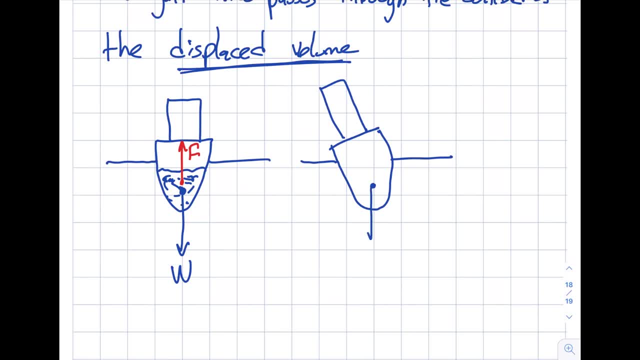 see this. the weight will still be over there. it will be like this, but the buoyant force due to the it's leading towards the left hand side over here. point force is now going to move like this. all right. so let's look at the next net effect. let's look at the moment. right, so what happens? 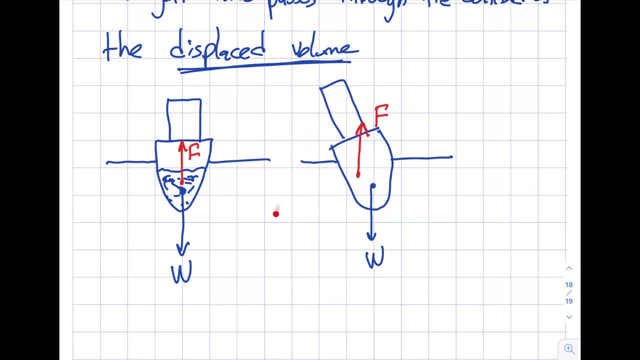 is the ship. if what it wants to overturn is, it needs to go this way, right. but look at this, how weight is. so now weight is stabilizing this, and actually look at the buoyant force: it's pushing it up so it goes back to the original shape. so that's why this is called hydrodynamically. 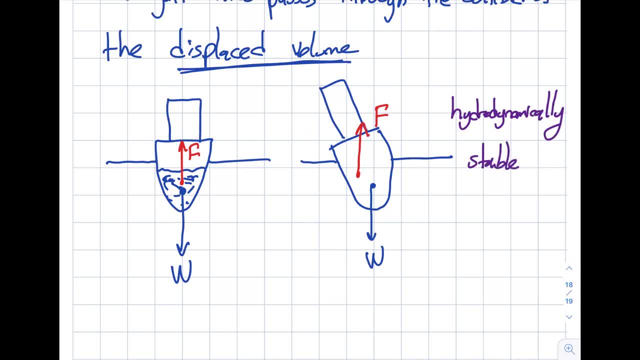 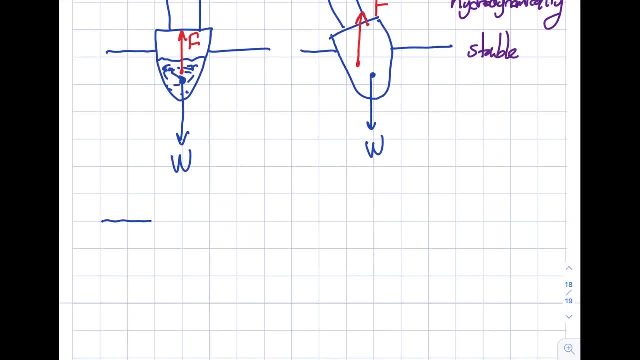 stable. so this is where you wanna be, okay. so now i will give you a second example. in the second example, what i do is you can think of this as, let's say, like this right, i'm trying to replicate the same and i have something like this right, but this time around. 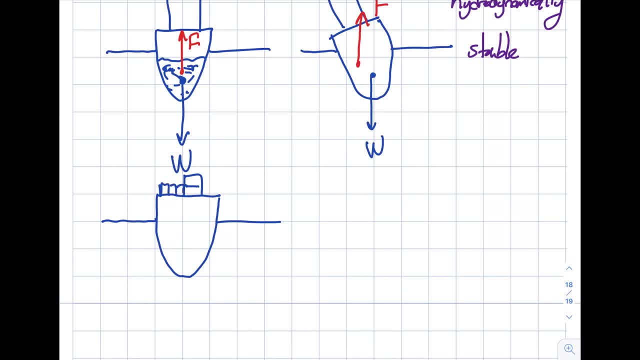 put a bunch of load up here. I have a bunch of load up here, I'm loading this up, okay, so what will happen is, if I have a bunch of weight over there, where the weight is applied will go up over here. so that will be W, but the buoyant force. 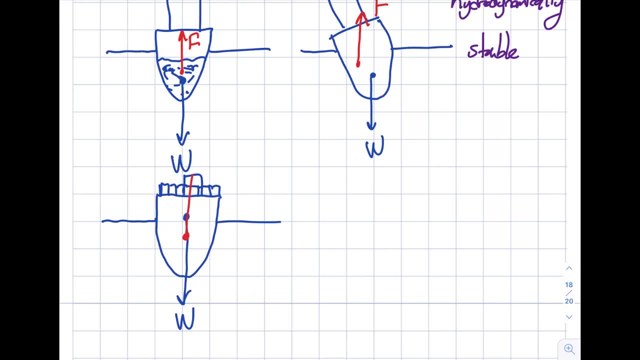 if you think about it, they are similar. now the buoyant force is gonna be like this: right, this is the F buoyant. so let's analyze this case when it has an angle to it because of the wind, and all right, let's say this is the water. 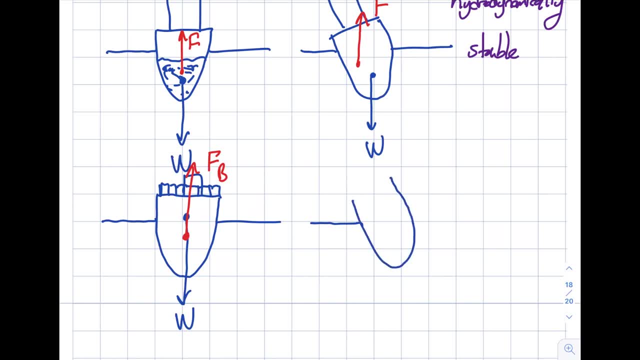 surface and I have some type of an angle over here. this is like that. this and I bunch of load over here. alright, now let's see this case. what happens is: now the weight is a pop. right. if the weight is up top now the weight is the center of the weight is going to move to this direction, right, so it's. 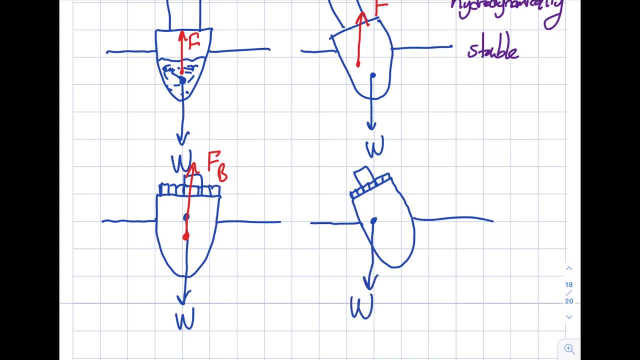 gonna be like this now, because look at the red weight, is the weight will be like that and then boiling force will be this way because think, take a look at it, it's the center of this place- fluid. so it's here, it's good, it's over here, not. 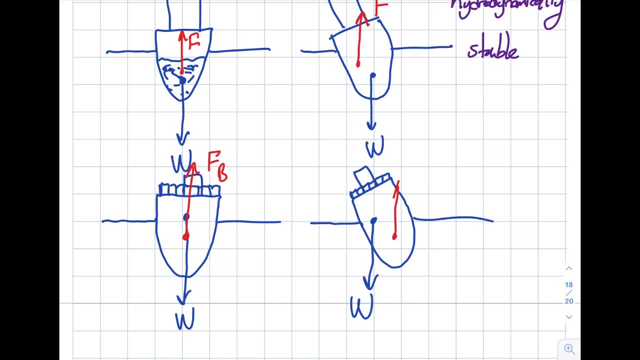 over there. okay, so then this will push it up. so now let's see what's going on the. the container now wants to go this way. right, you're trying to prevent it, but look at what the weight does: it also pulls me down. it will also pull me up. 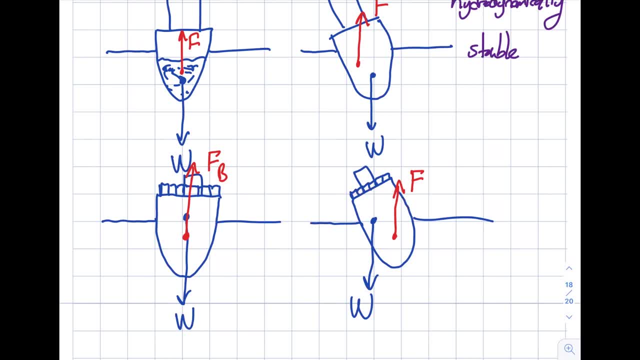 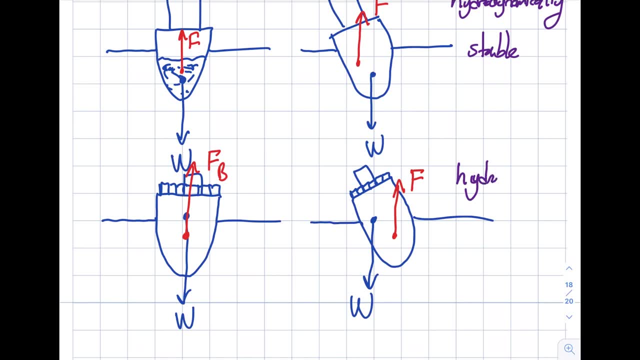 how about that? well, now F is also pulling it down over, so it can easily overturn. that's why to these things we call hydro dynamically unstable. okay, so this is important, this is unstable, this is stable, so you always want to put the load at the bottom. okay, now that the top top heavy is no good. you notice the. 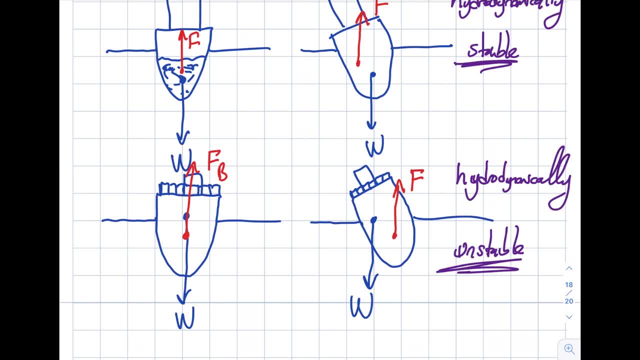 expression as well. it's top heavy right. so now in the next segment, I will solve a question or two to illustrate how these concepts are applied.